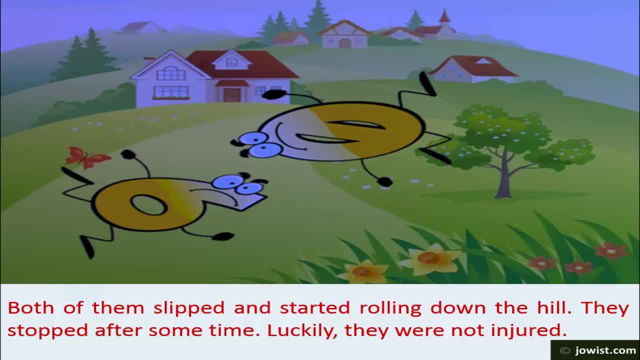 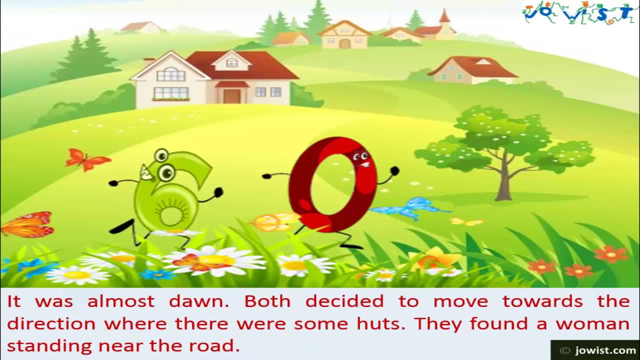 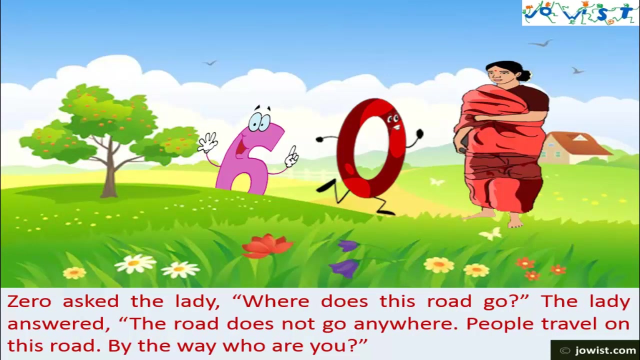 They stopped after some time. Luckily they were not injured. It was almost dawn. Both decided to move towards the direction where there were some huts. They found a woman standing near the road Zero. asked the lady: Where does this road go? 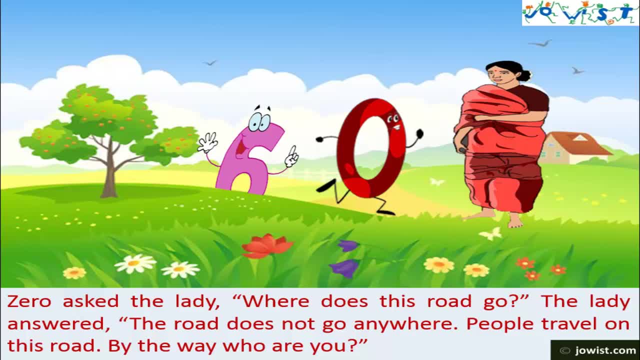 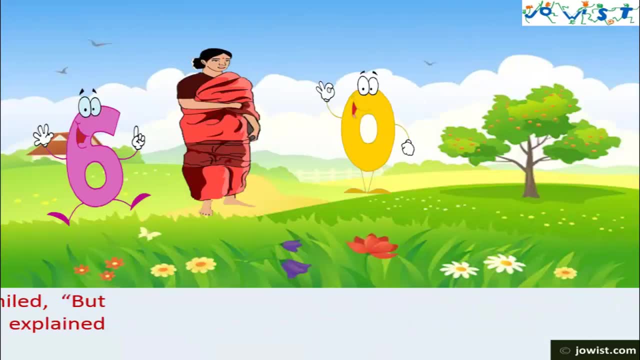 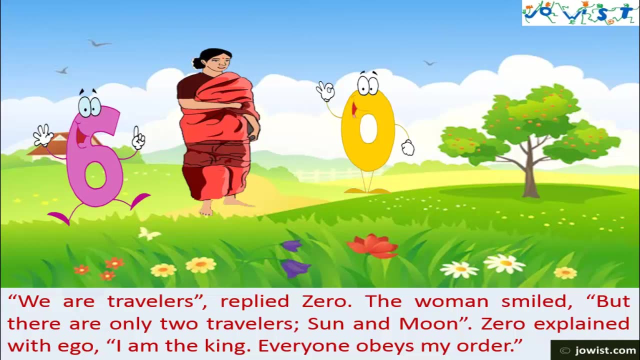 The lady answered: The road does not go anywhere. People travel on this road. By the way, who are you? We are travellers, replied Zero. The woman smiled, But there are only two travellers: Sun and Moon. Zero explained with ego. 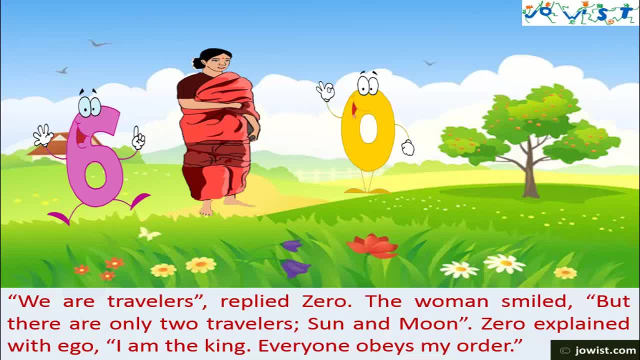 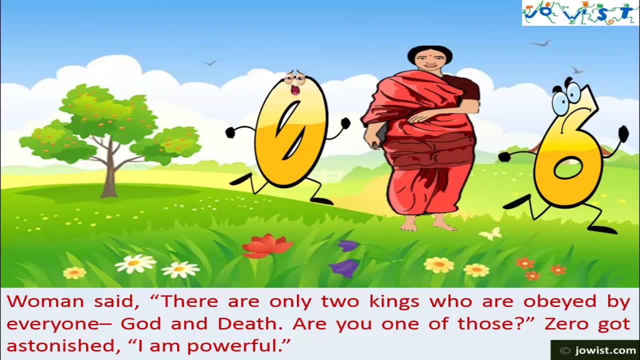 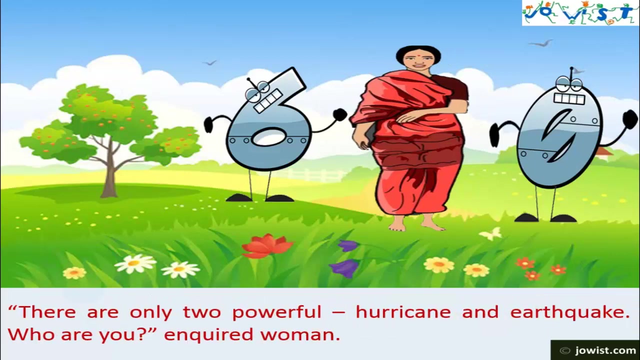 I am the king, Everyone obeys my order. The woman said: There are only two kings who are obeyed by everyone: God and Death. Are you one of those? Zero got astonished. I am powerful. There are only two powerful. 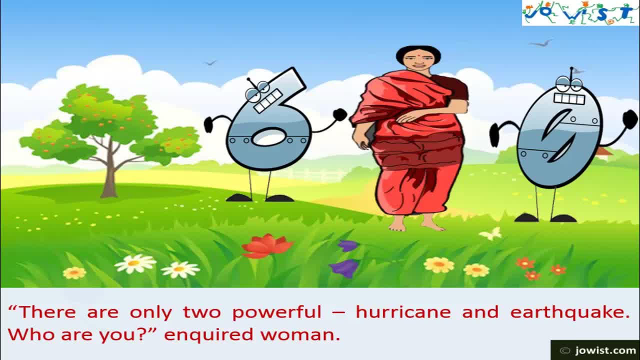 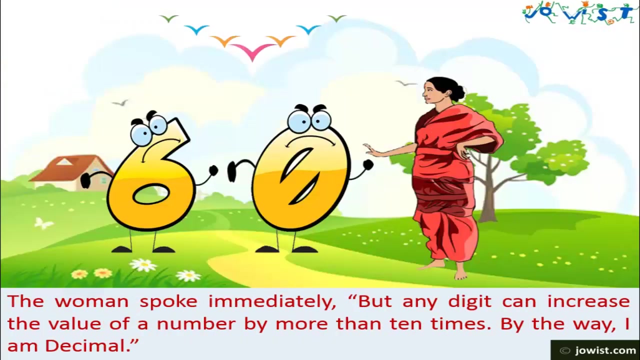 Hurricane and Earthquake. Who are you inquired? the woman, Zero in anxiety, said I can increase the strength of a number by ten times if I suffix them. The woman spoke immediately. But any digit can increase the value of a number by more than ten times. 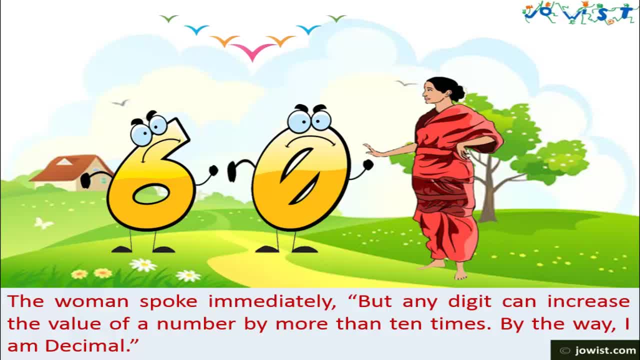 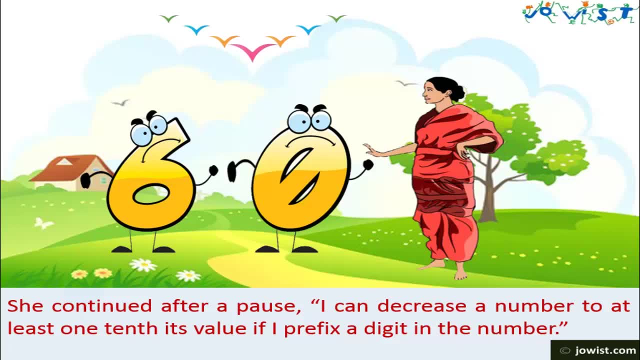 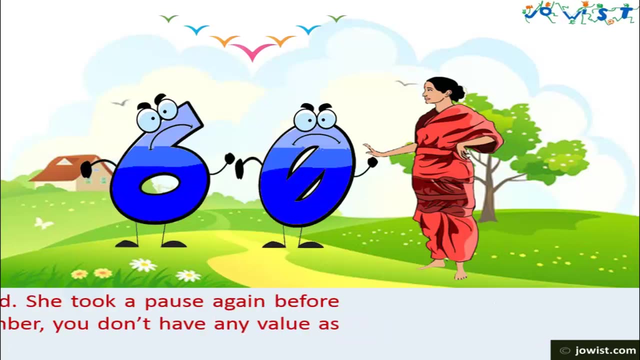 By the way, I am decimal. She continued after a pause. I can decrease a number to at least one-tenth its value if I prefix a digit in the number. Zero seemed to be confused. She took a pause again before she spoke. 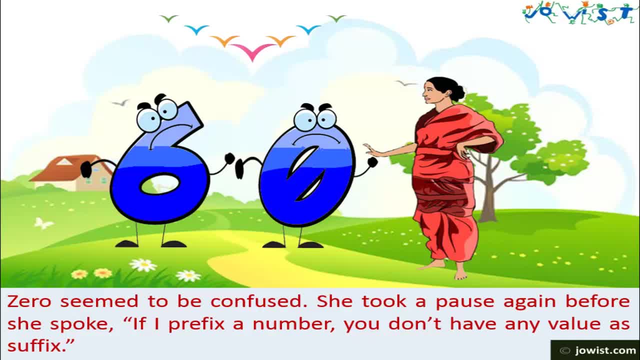 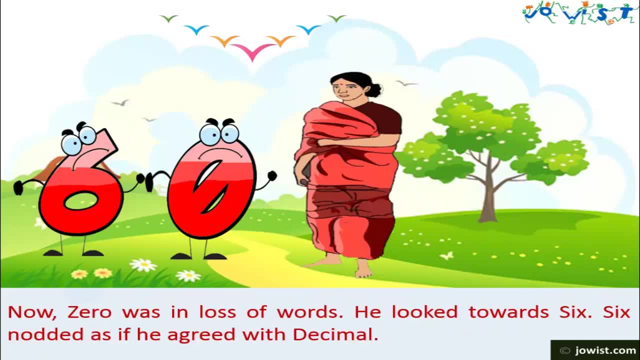 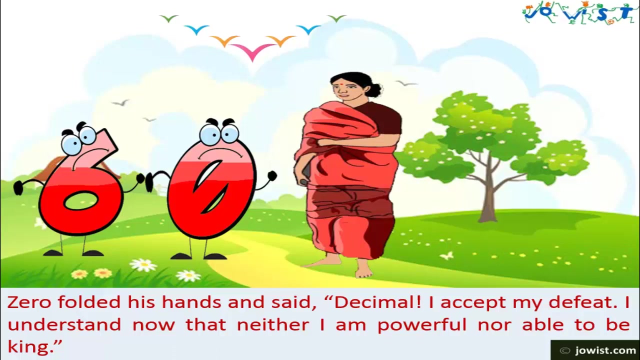 If I prefix a number, you don't have any value as suffix. Now Zero was in loss of words. He looked towards Six. Six nodded as if he agreed with Decimal. Zero folded his hands and said: Decimal, I accept my defeat. 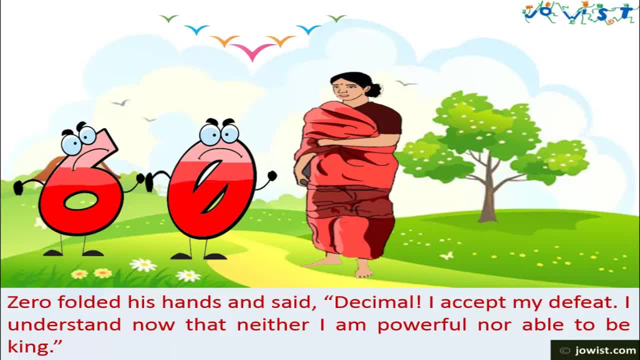 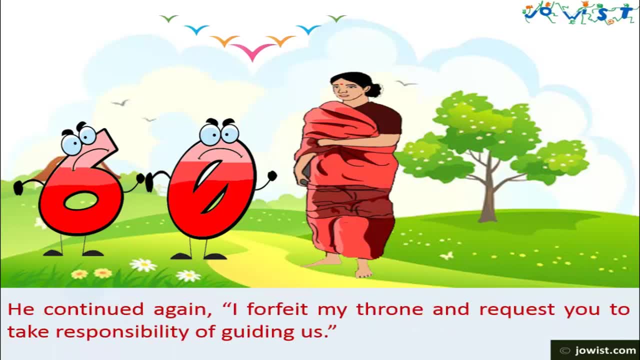 I understand now that neither I nor you can defeat me, That neither I am powerful nor able to be king. He continued again: I forfeit my throne and request you to take responsibility of guiding us. Decimal said: I am not willing to be a ruler. 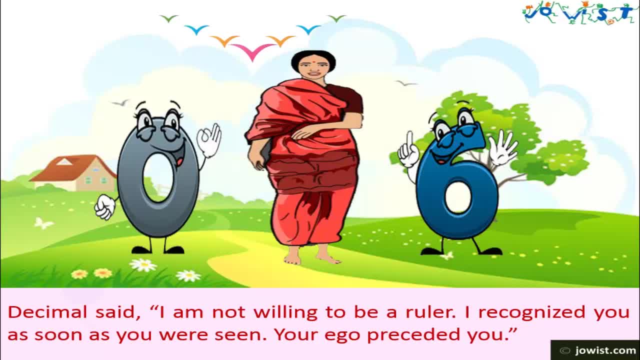 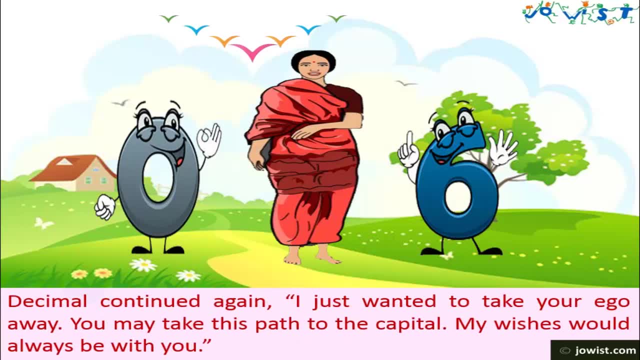 I recognized you as soon as you were seen. Your ego preceded you. Decimal continued again. I just wanted to take your ego away. You may take this path to the Capital. My wishes would always be with you. Zero and Six thanked Decimal and left for the Capital. 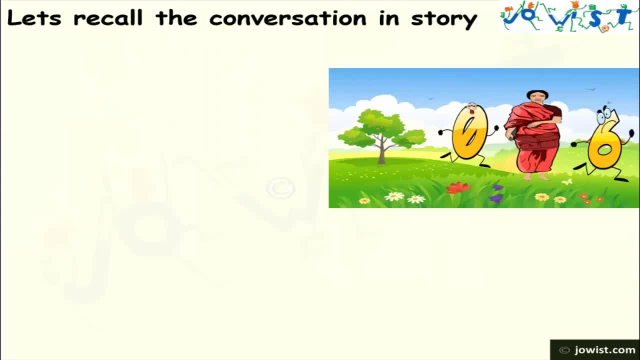 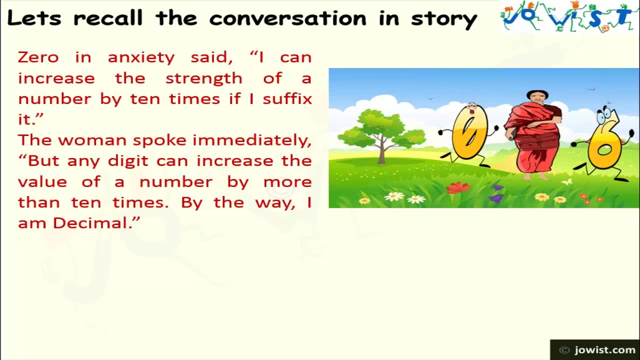 Now let's recall the conversation of Decimal and Zero. Zero, in anxiety, said I can increase the strength of a number by ten times if I suffix it. The woman spoke immediately. But any digit can increase the value of a number by more than ten times. 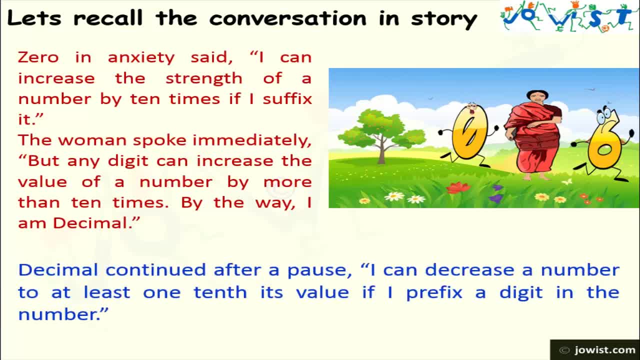 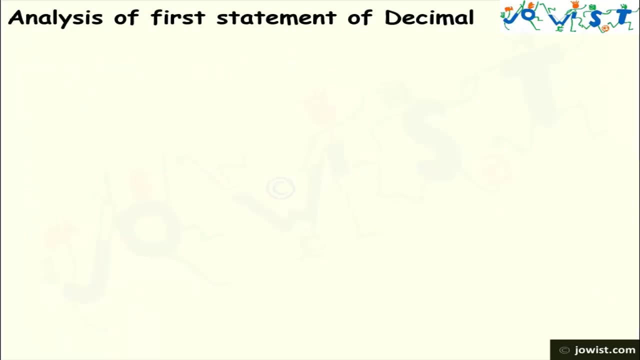 By the way, I am Decimal. Decimal continued after a pause. I can decrease a number to at least one-tenth its value if I prefix a digit in the number. Let's evaluate these statements. Let's evaluate the first statement which Decimal said. 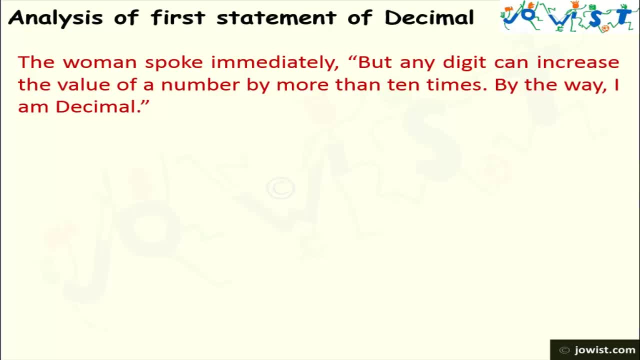 What did she say? She said: But any digit can increase the value of a number by more than ten times. So let's check it with an example. We take a number 35.. Let's put zero first. If we suffix zero, the number becomes 300. 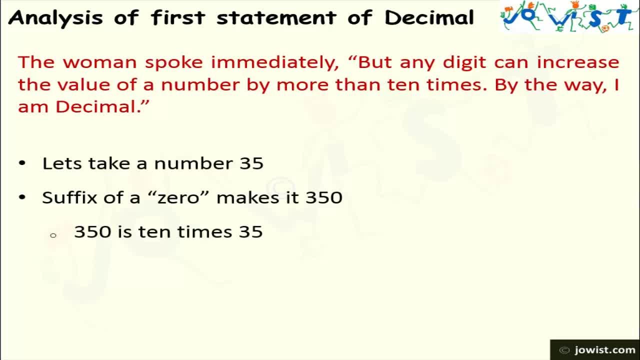 The number becomes 350.. 350 is ten times of 35.. Now let's try to suffix any other number apart from zero. Let's suffix eight. If we suffix eight, the number becomes 358.. Certainly, it is more than ten times of 35, isn't it?